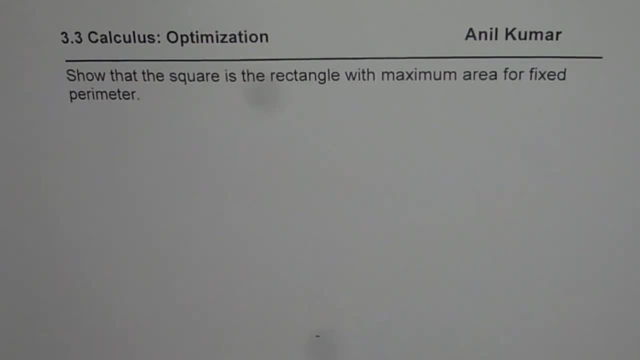 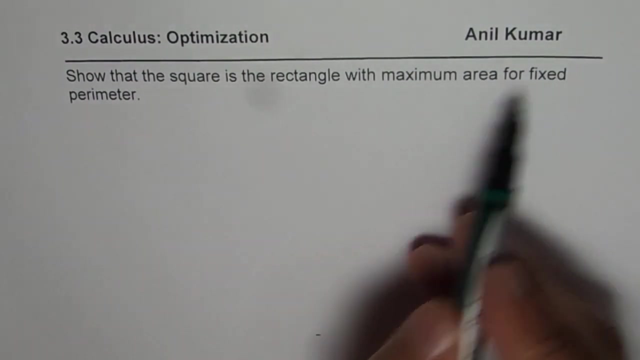 I'm Anil Kumar and with the help of this very general question, we'll get to know a very important thing on optimization. The question here is: show that the square is the rectangle with maximum area for fixed perimeter. You will come across many questions where we are given the perimeter We 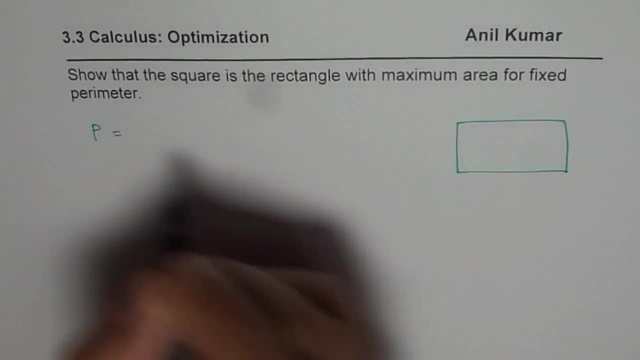 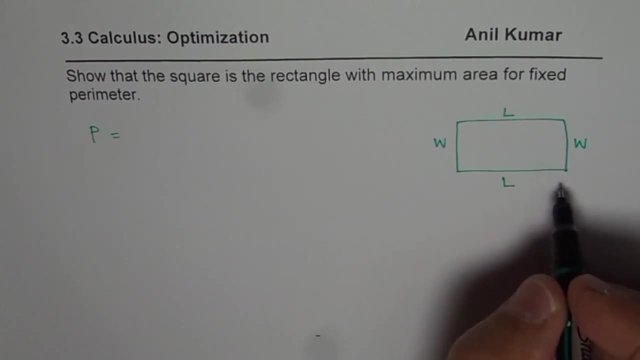 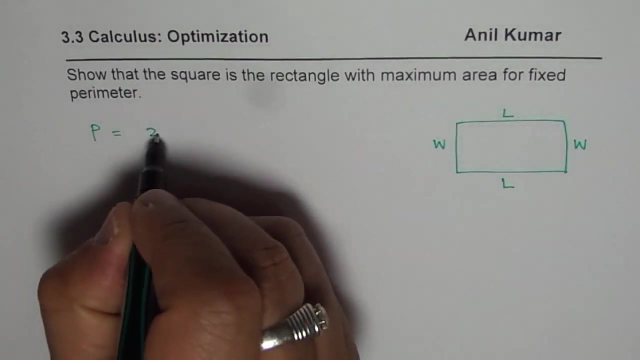 say perimeter is fixed, So we say p is fixed, Perimeter is what It is: sum of length and width of a rectangle, right? So let us say we have a rectangle in general. So when we say perimeter is fixed, that means constant. then it is normally equals to 2 length plus 2 width. right Now, if 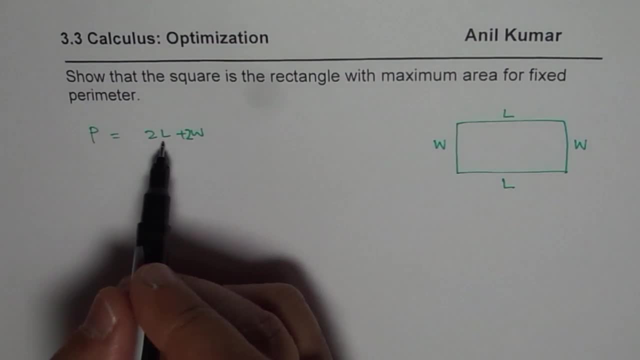 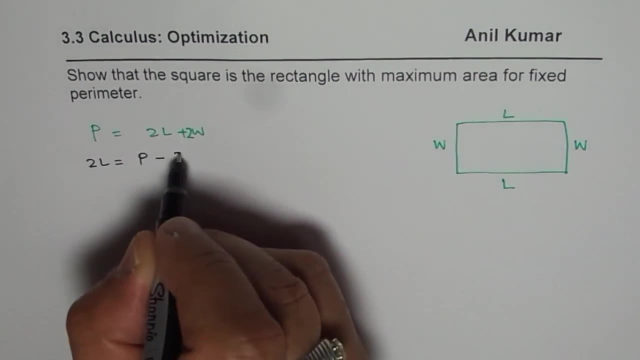 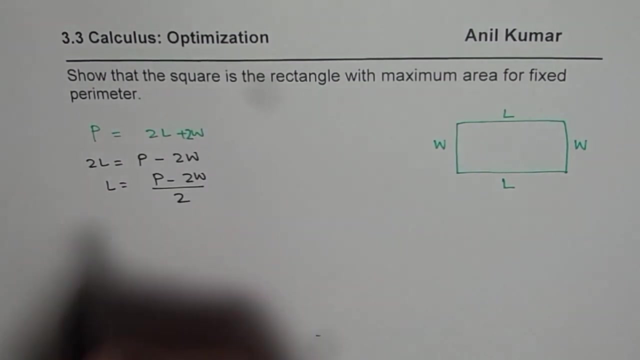 perimeter is fixed, then we can always write one dimension in terms of the other. So we say 2 length is equals to perimeter, Perimeter minus 2 width. or length is equals to perimeter minus 2 width divided by 2.. So we get. 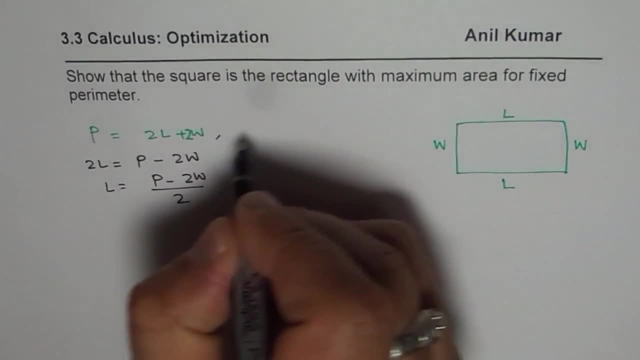 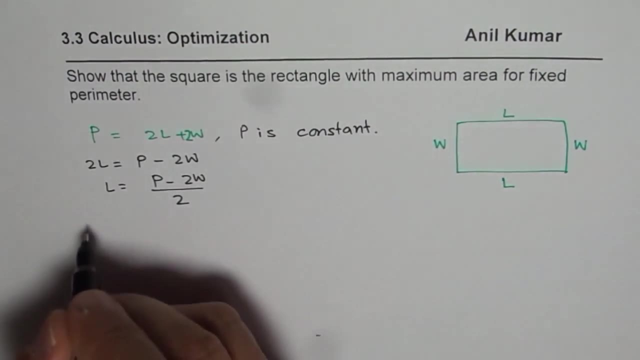 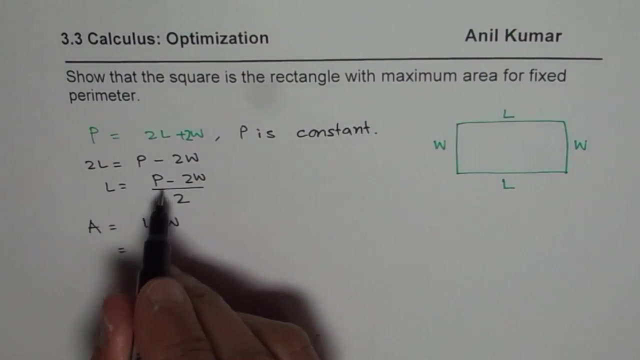 length in terms of width and perimeter, where we know perimeter is constant, Constant or fixed. right Now, what is area? Area is length times width. So now we know length in terms of width will substitute p minus 2w Over 2 for length times width. So what we get here is an expression which is only in w, So we can. 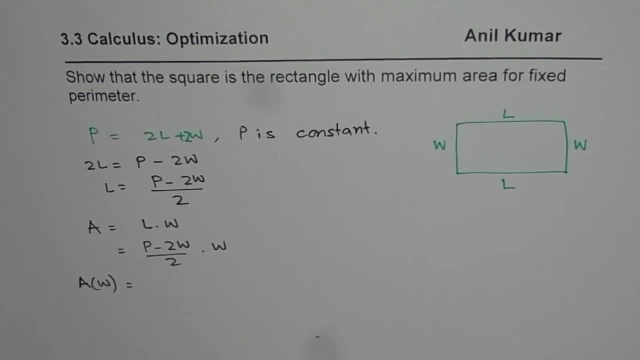 write this as area, in terms of as a function of width, You get the point right Now here. if I multiply this, then what do I get? I get pw over 2.. Let me write them separately. Minus 2 and 2: cancel w square. 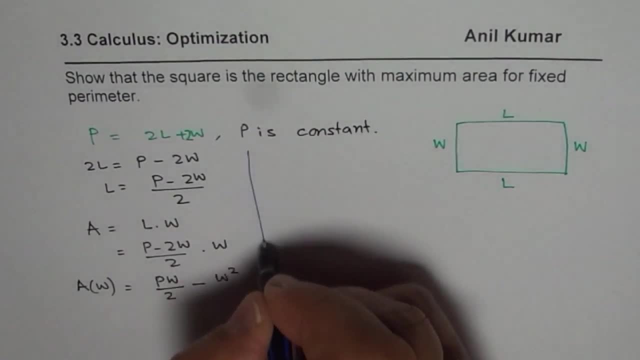 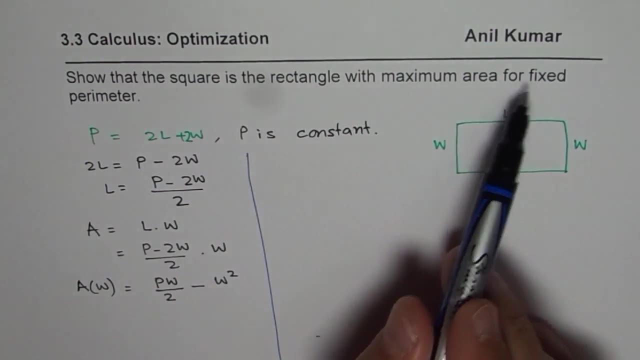 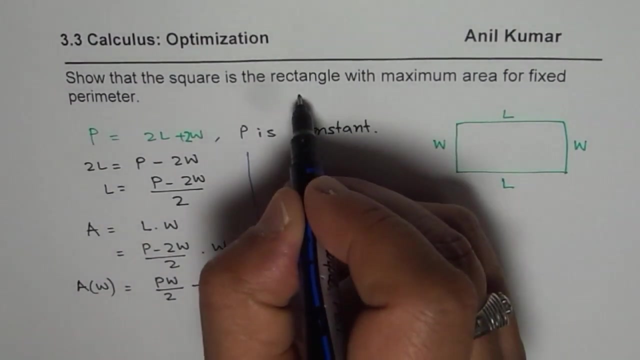 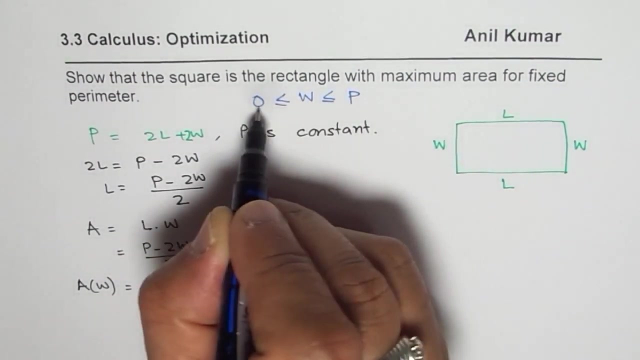 That is an expression which we will get Now. the question is: show that this square is the rectangle with maximum area for fixed perimeter. Now, if perimeter is fixed, then length and width, how are they related? We can say that width can maximum be equal to perimeter and least it will be 0.. So 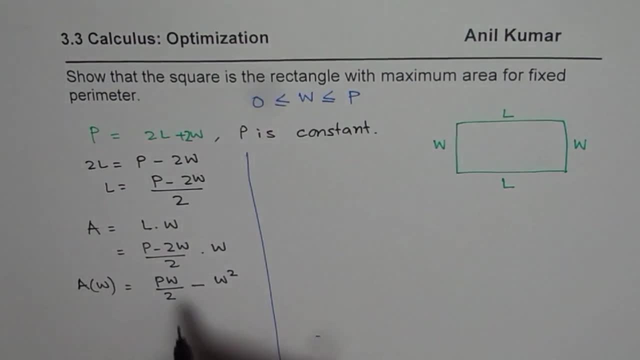 those are the boundary conditions for the width we can find using derivative right. So we can equate derivative of area to 0 to get our critical number right. So let us find the critical number now, So a. let us write a w. 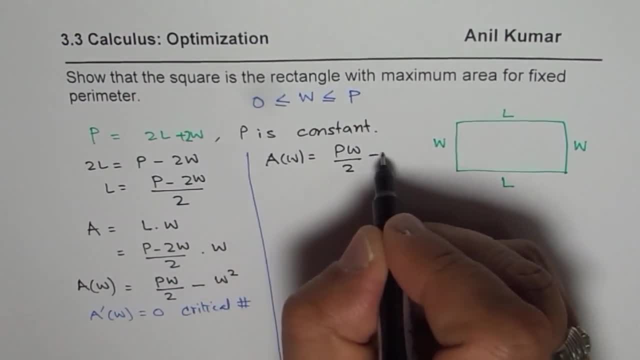 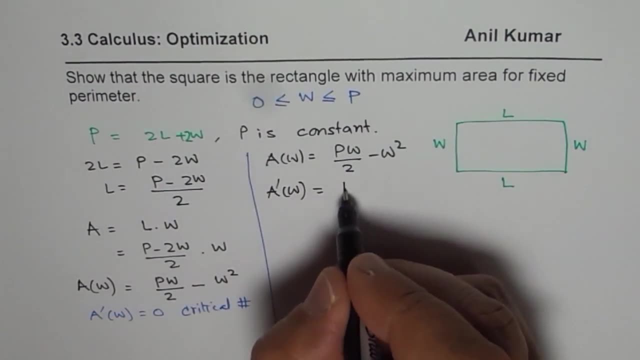 equals to p w over 2, where p is constant w square. So a dash rate of change of area with width will be p over 2 minus 2 w right, And this is 0. That means p over 2 minus 2 w should be. 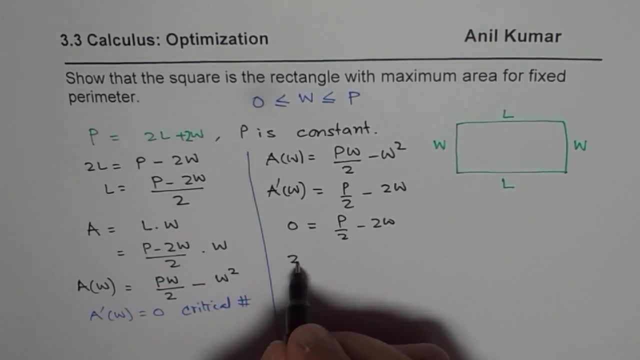 equal to 0.. From here we can solve: for w We have 2, w equals to p over 2, or width is equals to p over 4.. Now, if width is p over 4, what is length? Let us find out. 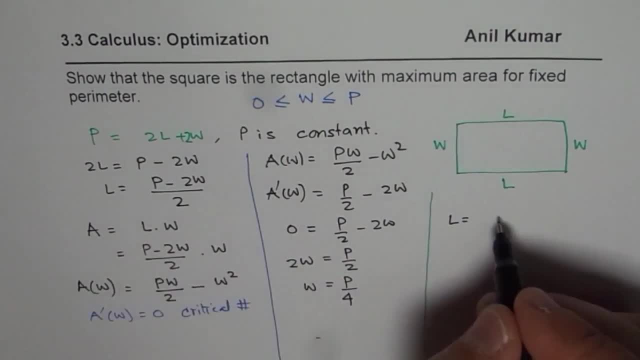 Length is equal to perimeter minus 2 times width. Width is p over 4, right Divided by 2.. So which is equals to p minus p over 2 divided by 2, right, So that is half p. So that is p over 2 divided by 2, or. 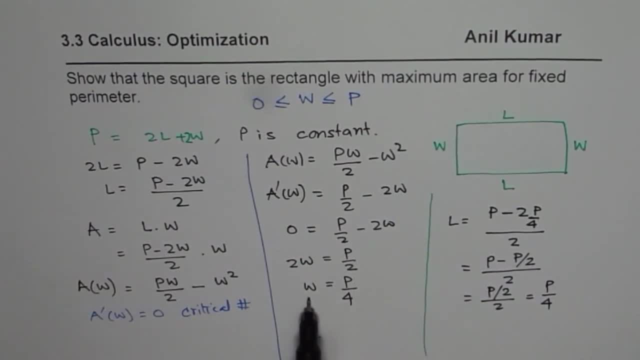 p over 4.. So what we notice is both length, width and width are same, So that means the structure is a square right. So what we get is: for maximum area, width equals to one fourth of perimeter and length is also equals to. 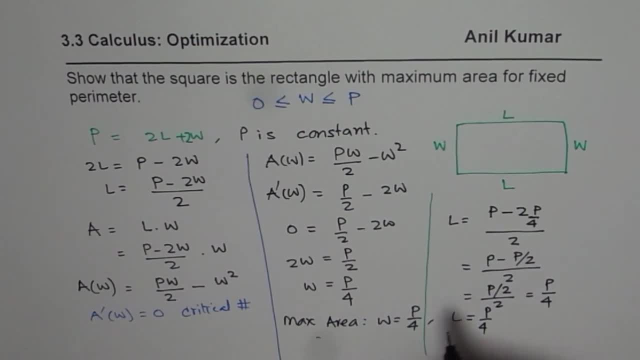 one fourth of perimeter. So since both those sides are equal, it is a square. So, in general for any given rectangle with fixed perimeter, if you need to find what are the dimensions of the rectangle for maximum area, The answer is square One. 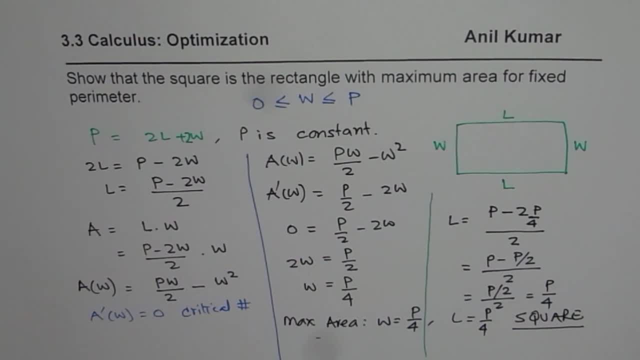 fourth of perimeter is the side of your square. I hope that helps. Thank you.